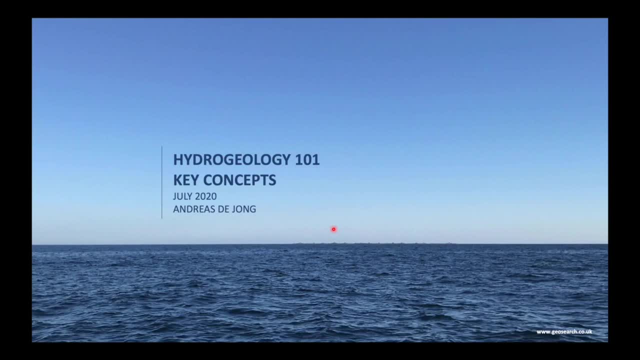 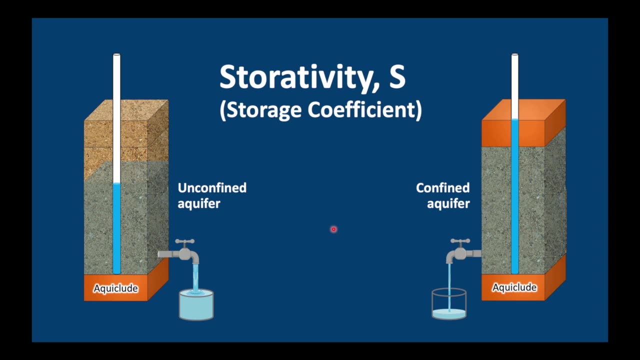 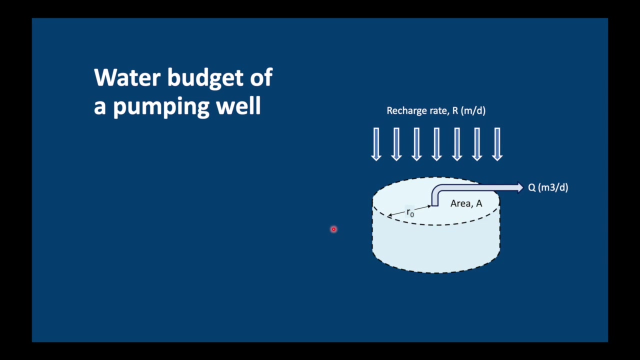 Welcome to Hydrogeology 101: Key Concepts. Today I'd like to talk about storitivity, also known as the storage coefficient. In a previous video we talked about the water budget of a pumping well and we said that if the discharge is balanced exactly by the recharge, then we might reach steady state. 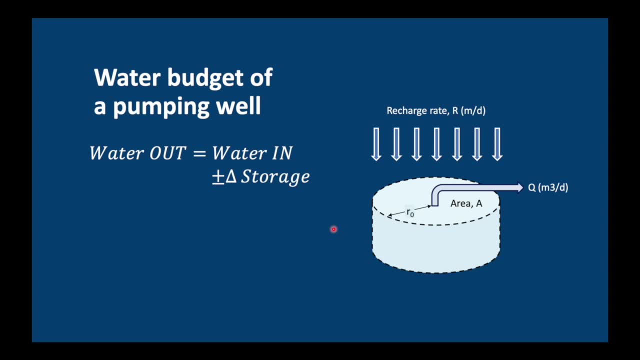 In most situations, however, the amount of water leaving the system is not the same as the amount of water coming in, and the equation has to be balanced by a change in storage. Think of it this way: Every month you're going to spend some money, and every month you have a. 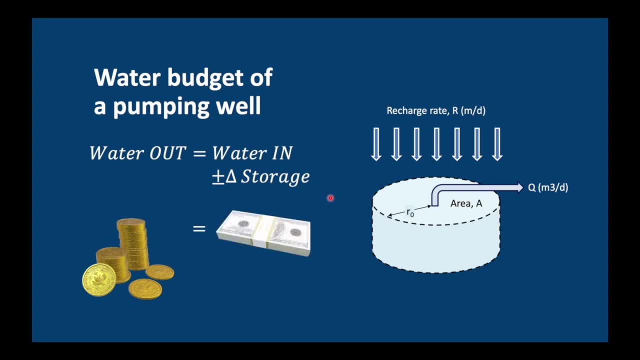 paycheck. If you spend more money than you receive through your paycheck, then you're going to have to take money from savings. If you're lucky and you spend less money, then your income, of course your savings pot, will grow. So, in a way, 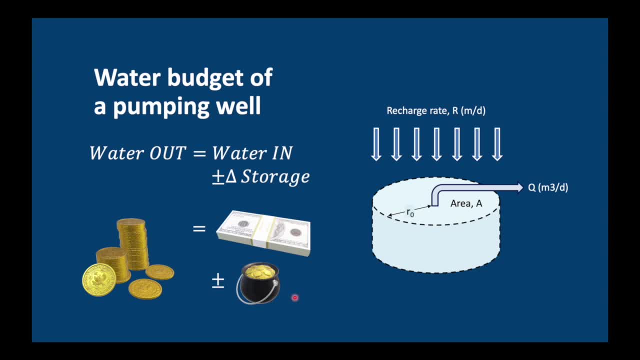 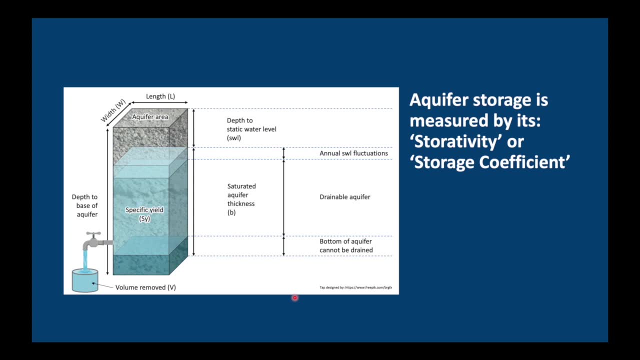 our storage coefficient is balanced by a change in storage, And storage is similar to our savings. ACFA storage is measured by the term Storativity or storage coefficient. From now on, I'm just going to talk about storitivity so that you don't get confused. 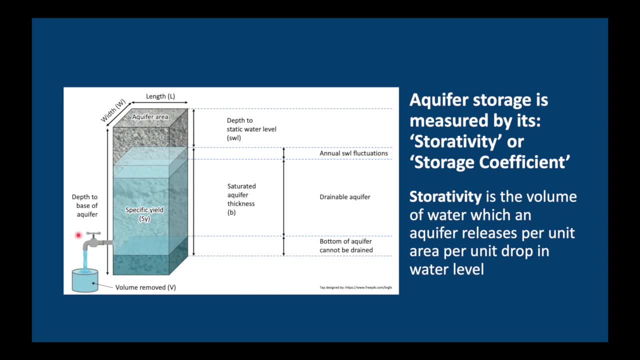 Storitivity is the volume of water which an ACFA releases per unit area, per unit drop in water level. That means that the storitivity of an ACFA is really important if we're going to do any kind of water budgets or aquifer resource assessment. 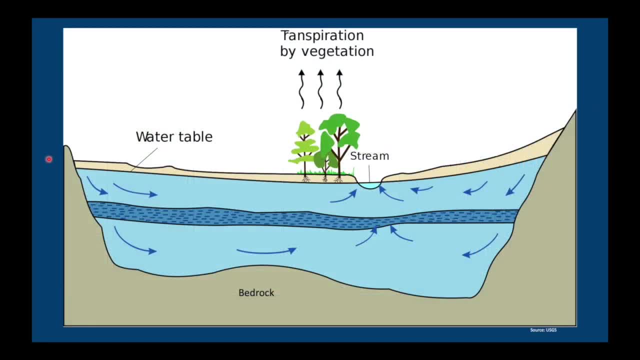 and so on. Here's a diagram of an alluvial aquifer. You can see this nice stream here, a water table, and the top part of it is an unconfined aquifer. That means that if we were to drill a water well at this location, then 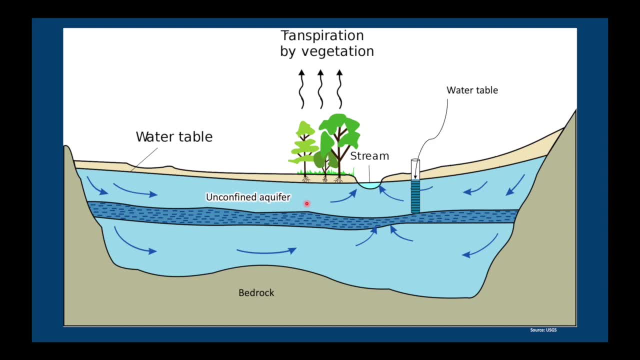 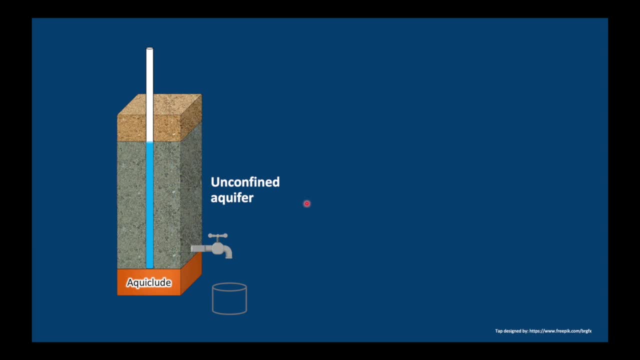 the water level in our well will be the same as the water table. This is what a piece of this unconfined aquifer might look like, with an original water table here and a well shown here, with a water level at the water table. 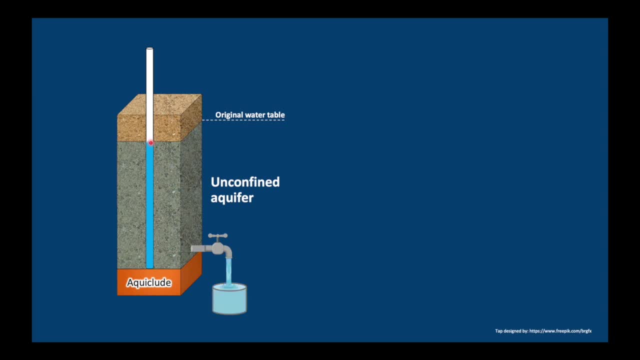 Now, if we start pumping water from this aquifer, which means we're extracting water, the water table will drop by a certain amount. This means that an unconfined aquifers groundwater is released from storage by de-watering of the aquifer. 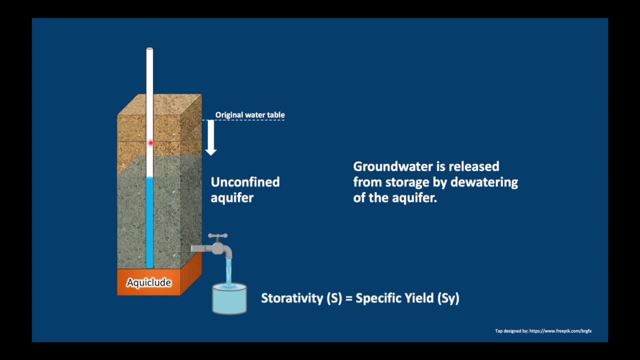 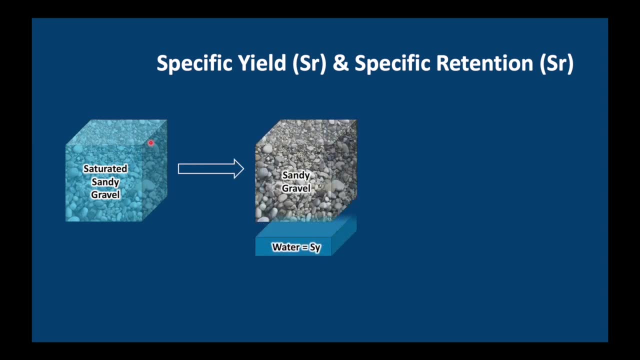 The storativity of unconfined aquifers is the same as the specific yield. In a previous video we saw how a certain amount of water can be abstracted from a saturated sandy gravel by drainage. That's called a specific yield. Some of 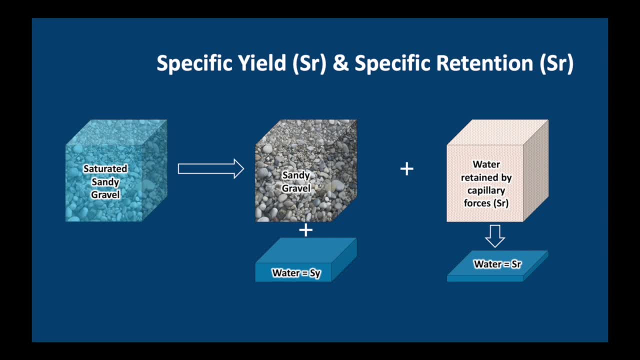 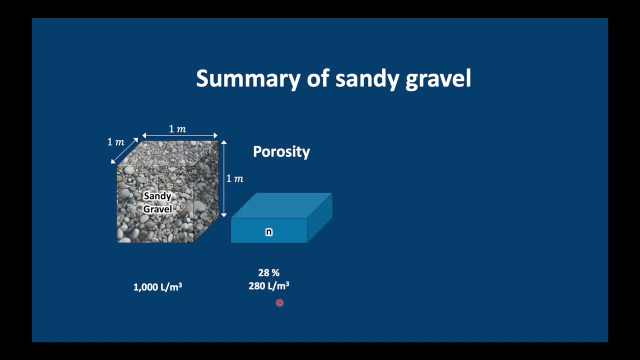 it also stays behind, which we call specific retention, And we did an experiment which showed that the sample of sandy gravel which had collected from the river had a porosity of 28%, a specific yield of 23% and a specific retention of 5%. I'd just like you to remember this rather large number here. 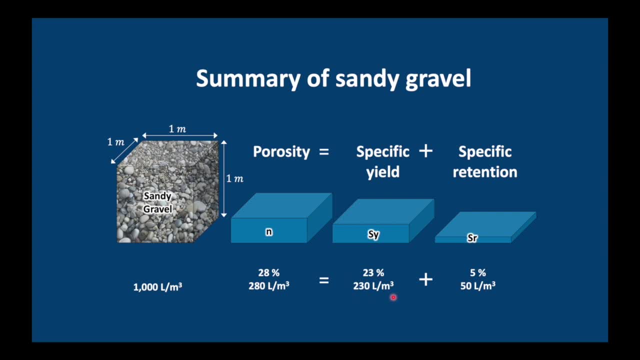 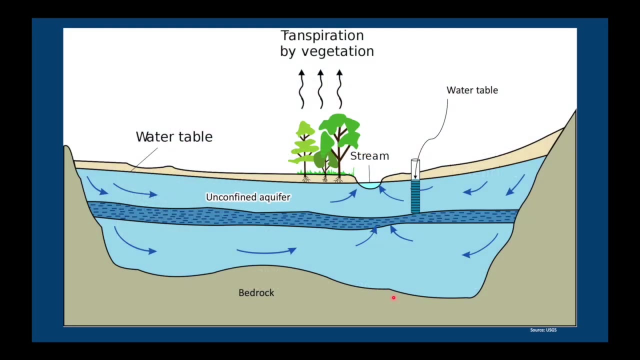 So from each cubic meter of sandy gravel we could drain 230 liters of water. So that's the storativity of this sandy gravel Aquifer under unconfined conditions. Okay, so let's say that we have a low permeability unit here. maybe some clays. 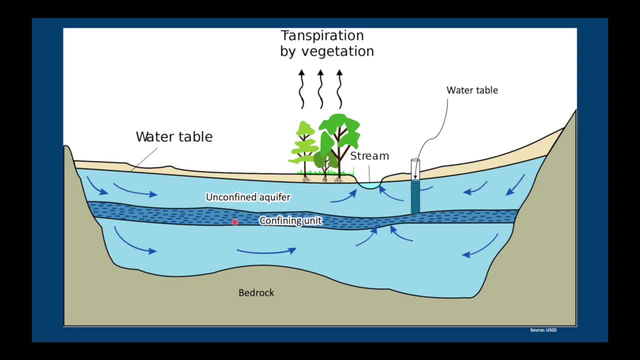 and this is acting as a confining unit to the confined aquifer below. Confined aquifer means that if we were to drill a water well down into this aquifer and seal it off properly so that it's only screened in the confined aquifer below, 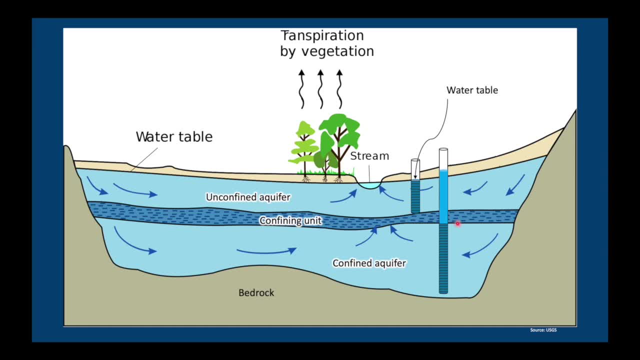 then our water level will rise inside the well up to a level which is equivalent to the piezometric surface of the confined aquifer. So that's just a precious surface and you can only see it from observation wells which are drilled into the aquifer. 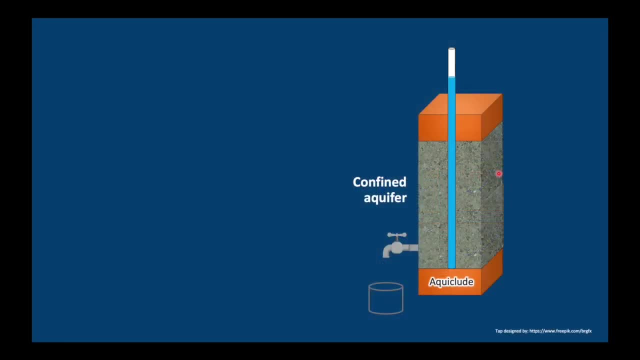 Ok, so here's a picture of our confined aquifer. It is sandwiched above and below by aquicludes and you see, here is our well, with the original piezometric surface shown here. Now, if we were to start pumping water out of this confined aquifer, what will happen is that: 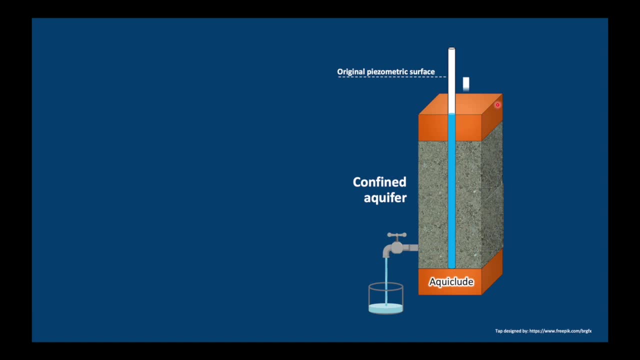 the piezometric surface will drop by a certain amount. Notice that the aquifer remains fully saturated. It will not be dewatered. Otherwise, it's not a confined aquifer anymore. This means that the groundwater is released from storage by depressurization of the aquifer. 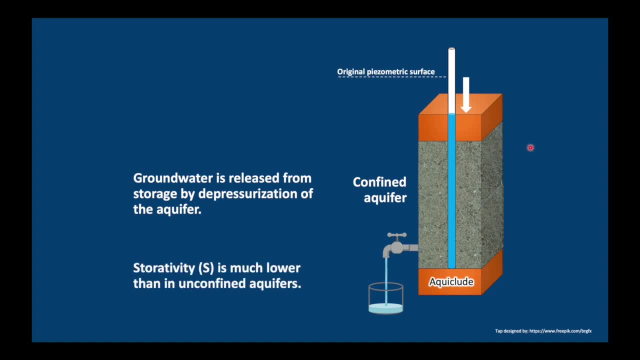 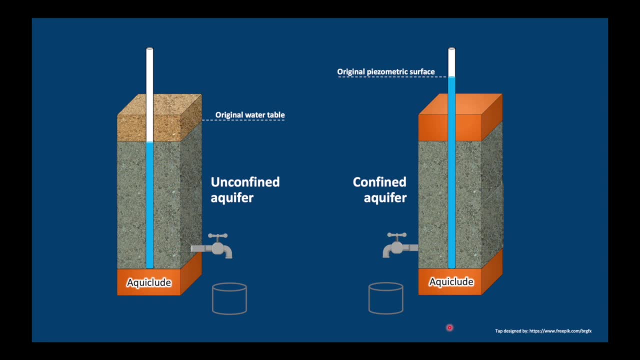 The storativity is much lower than in unconfined aquifers. I've tried to show that here by a small amount of water in the pot. So just to recap: in unconfined aquifers our storativity is the same as the specific yield. 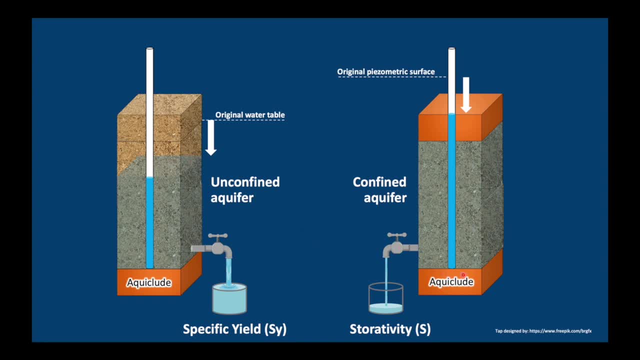 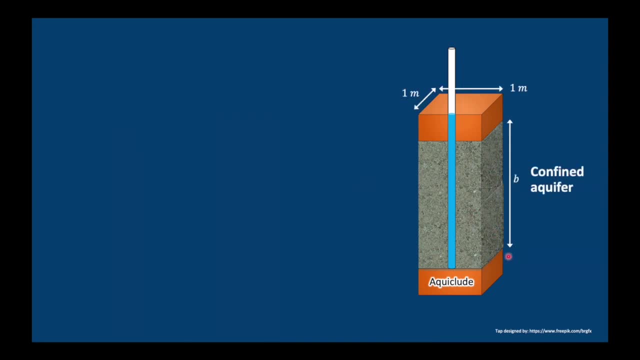 It's due to dewatering of the aquifer, And in confined aquifers, our storativity is only due to depressurization of the aquifer. Okay, so let's have a closer look at our confined aquifer. Let's assume that we have. 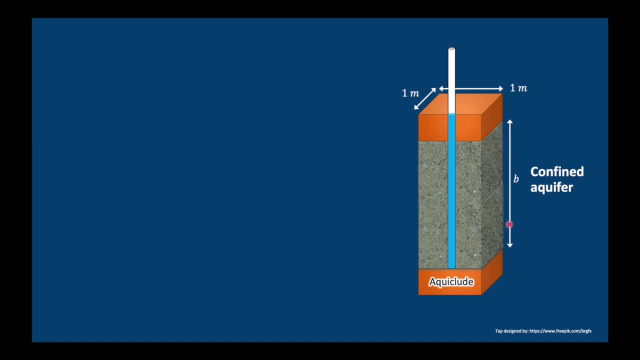 a 1 by 1 meter section of aquifer with a thickness b And we take out a cubic meter of this aquifer and we depressurize it by one meter, Then the amount of water which will be released from this one cubic meter of aquifer is called the specific storage. 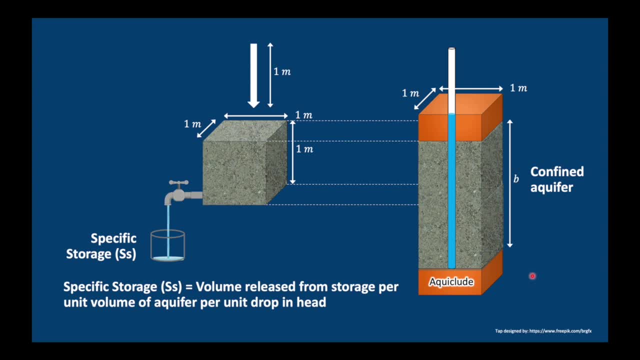 Specific storage is the volume released from storage per unit. volume of aquifer per unit. drop in head. So that means that we have volume in cubic meters, the volume of the aquifer also in cubic meters and the drop in head in meters. So cubic meters divided by cubic meters divided by meters, and we end up with this. 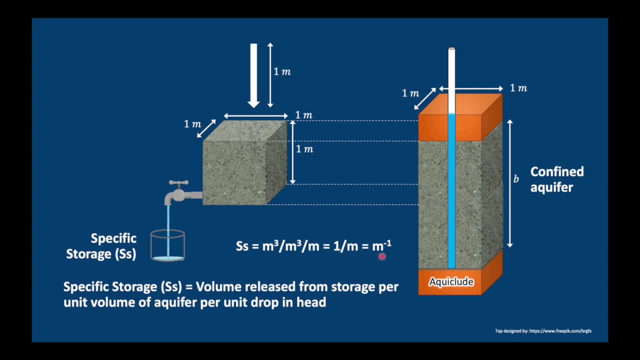 funny unit here, which is meter to the minus one One over meter. Okay, now let's have a look at our aquifer as a whole. If we drop the pressure here by one meter, then the total amount of water which we can abstract from the aquifer- 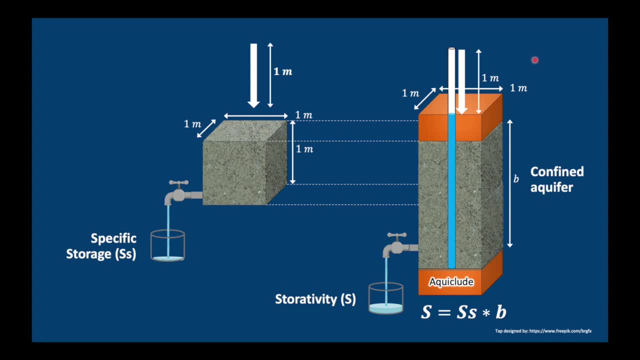 is called the storativity. The storativity is a specific storage times by the aquifer thickness And in words it is the volume of water released from storage per unit. So the volume of water released from storage per unit drops to the surface area, so that's one square meter here. 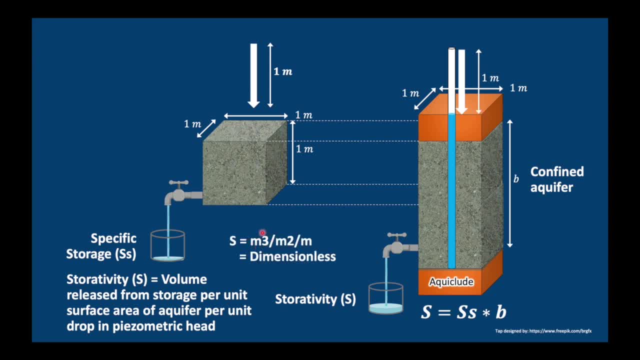 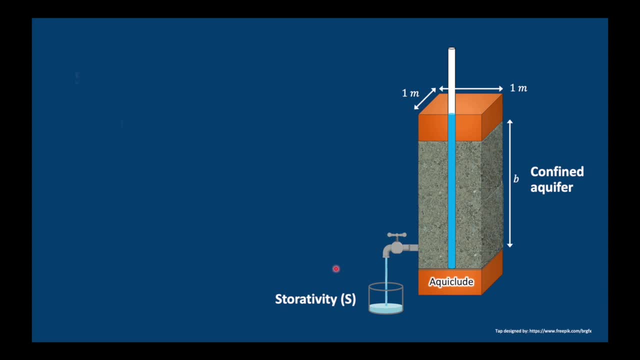 Per unit drop in piezometric head, which is one meter drop. So we have here dimensions of cubic meters divided by meter squared divided by meters. so basically it becomes dimensionless. Here are some normal storativity ranges in confined aquifers and you'll see it goes from about ten to the minus five to ten to the minus three. 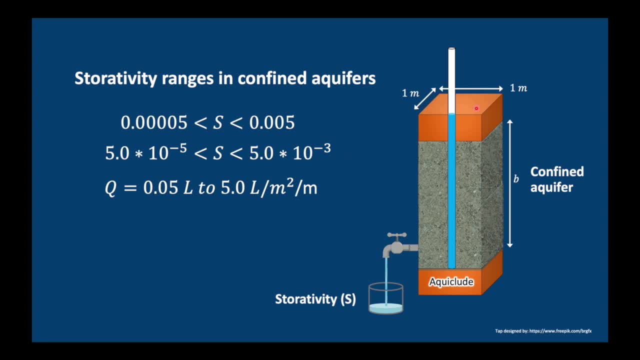 And the only difference in real terms is that from each square meter of aquifer and the one meter drop in pressure, you can only get about point zero. five liters to a maximum of five liters, So that's not a lot of water. to consider how much we could drain from our 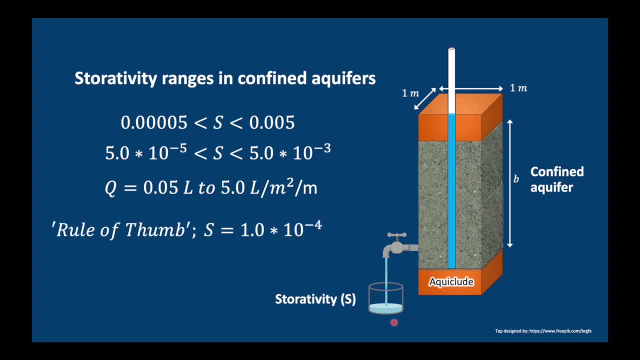 unconfined aquifer. If you don't know what the storativity is of a confined aquifer, just assume it's ten to the minus four. Another rule of thumb is that you take three times ten to the minus four, times ten to the minus four. 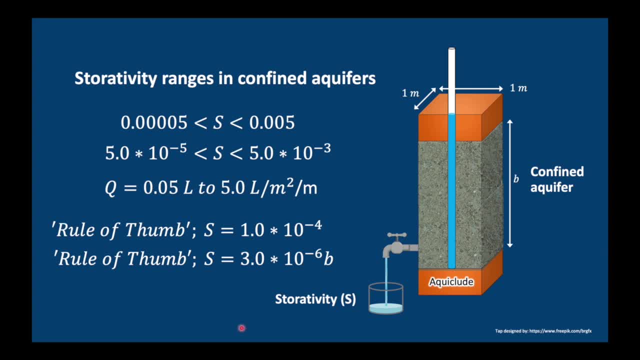 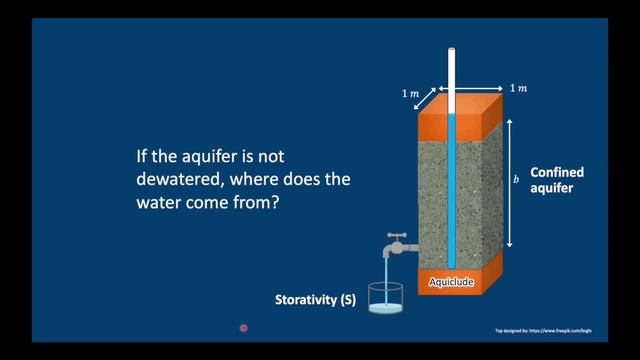 minus six and times it by the aquifer thickness. But basically, this is something you're going to have to work out in whatever part of the world you're in. Okay, if the aquifer is not dewatered, where does the water come from? 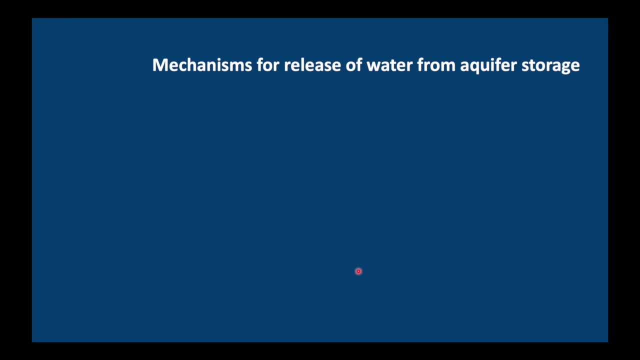 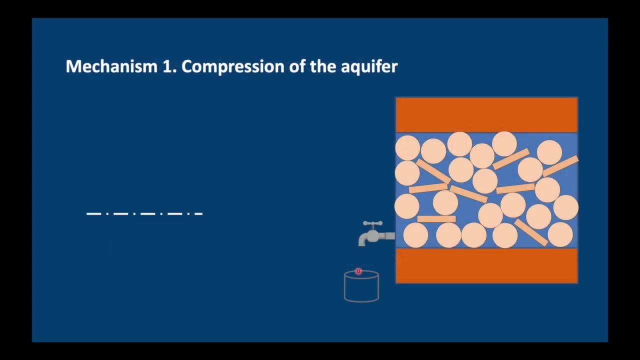 That's a good question. There are two mechanisms for the release of water from aquifer storage. The first is the compression of the aquifer and the second is the expansion of water. Let's look at the first mechanism first. Imagine that we have here a plane at the top of our aquifer. 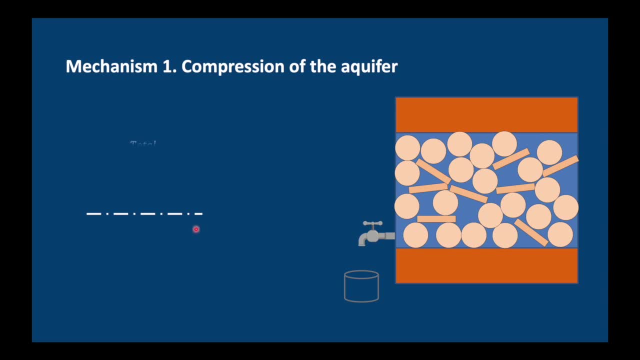 represented by this line here- Then the weight of all the material above this plane, that means all the sand and gravel and clays and water and whatever is above our aquifer- will be pushing down and that is called the total stress. Of course it will be met by the 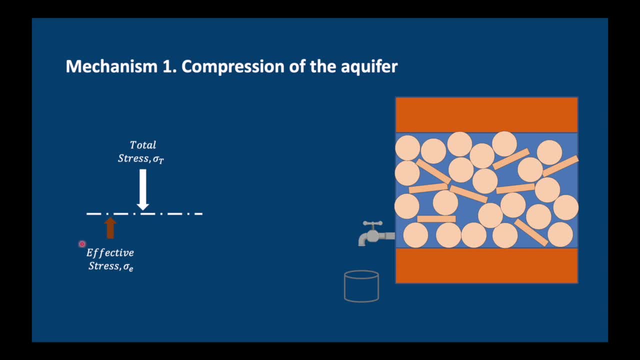 effective stress, which is the amount of stress that is borne by the aquifer materials themselves, plus the amount of stress that is borne by the pore fluid themselves. So that means the water in our aquifer is also supporting some of this overburden weight that's pushing down on the aquifer from above- Our total stress. 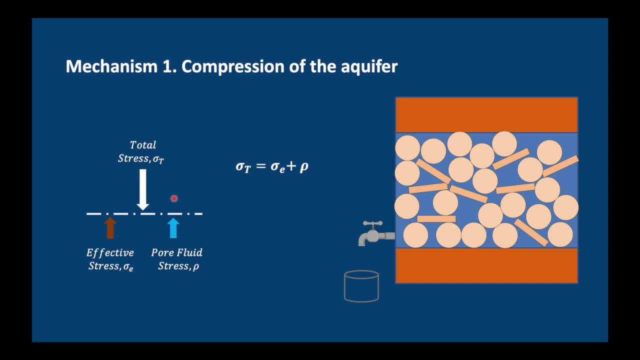 is always equal to our effective stress plus the pore fluid stress. So forces acting down are balanced by forces acting up. Let's have a look at our aquifer. here I've got some downward arrows indicating the total stress and the effective stress which is being borne by the aquifer material itself and the pore. 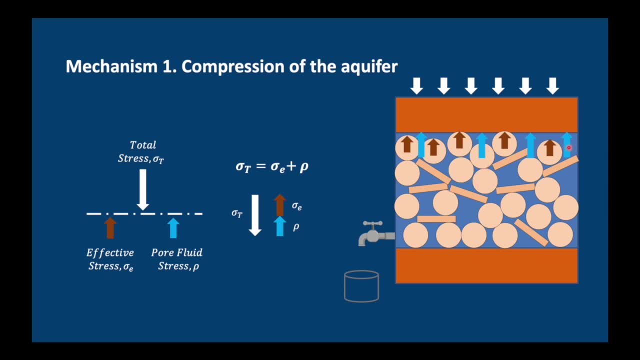 fluid stress which is acting upwards from within the water in our aquifer. Let's say, we start to pump water out of this aquifer. What happens? Well, we're going to reduce the pressure here of the pore fluid, which means that 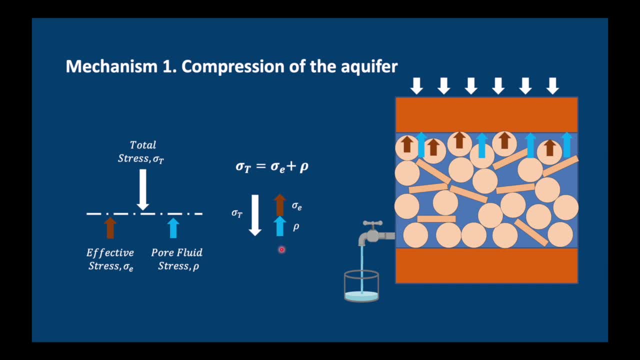 the pore, fluid stress will decrease. Because this equation has to balance, there's only one thing that can happen, that is, the effective stress has to go up. Basically, the aquifer material will have to bear more of this overburden load. And as there's more stress on our aquifer, 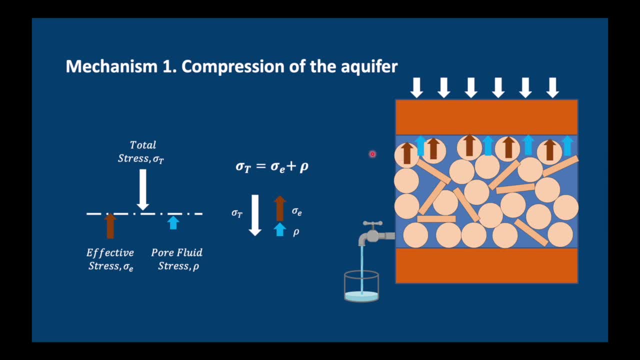 material, we might get a bit of compression of the aquifer. This reduces the pore spaces here and releases more water from storage. You'll notice that here the pore fluid pressure has decreased and it's been balanced by an increase in the effective stress. 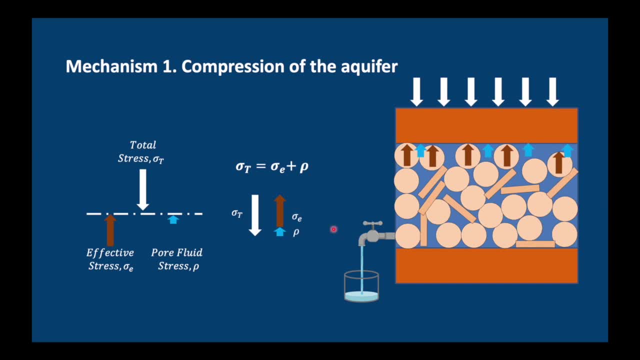 Okay, if we continue this process, you can see that the pore fluid stress is decreasing and the effective stress is increasing, and our aquifer is sorry. the voids in the aquifer are reducing in size, thereby releasing more water to our 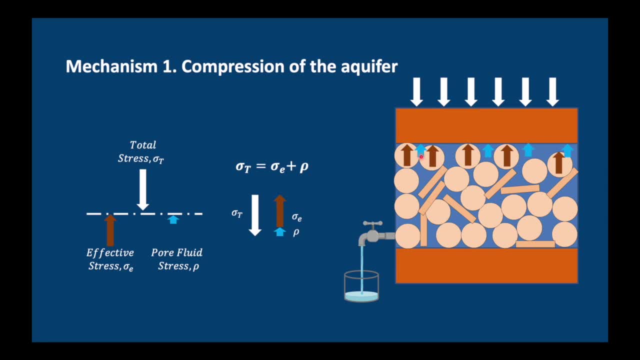 pumping well. Another thing that could happen is that the reduction in the pressure of the water- here the pore fluid stress- will mean that some of these particles might swell a little bit. This is particularly for clay minerals, maybe not so much for sand. 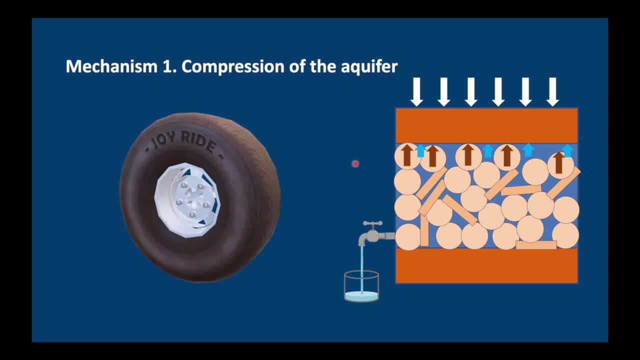 particles. Think of a confined aquifer like a car tire. You can let some of the air out, but that doesn't mean that the tire will be completely flat. It also means that we can, of course, pump air back into our tire and pressurize it again, the same as we. 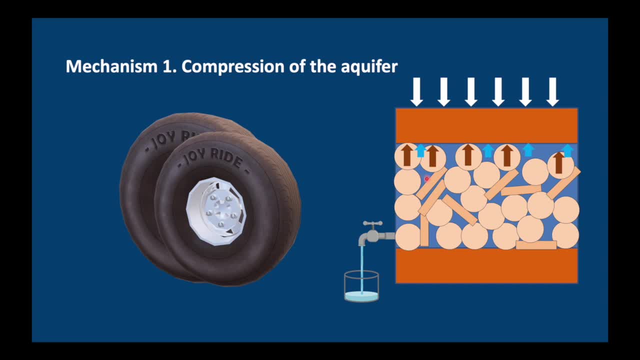 can put water back into our confined aquifer and increase the pore fluid pressure in here. Now we measure the compressibility of our aquifer in terms of this parameter alpha here, which is the change in volume over the change in stress. so that's that here is the effective stress And it is measured by the 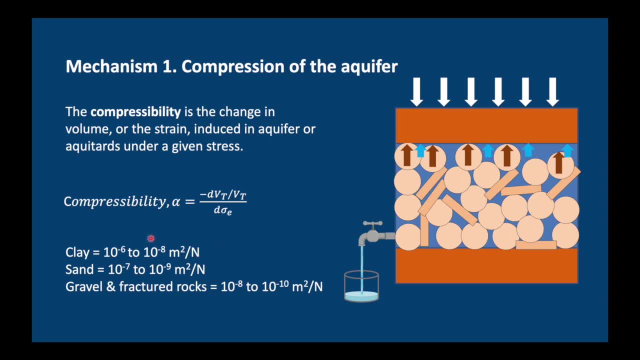 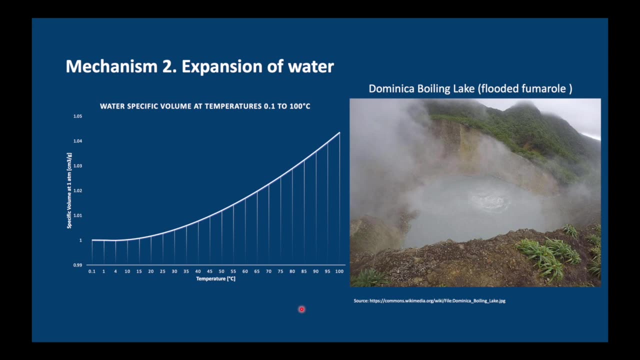 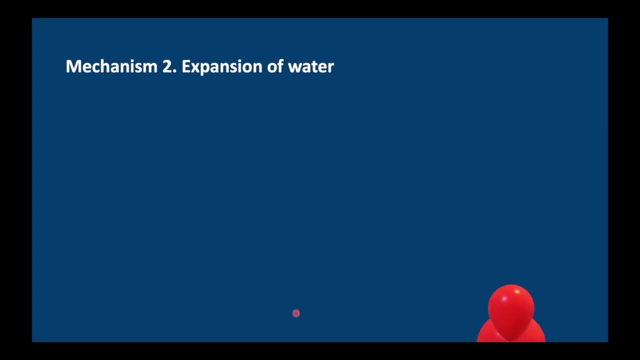 in units of meters squared per Newton, and you can see that clays are much more compressible than sand or gravel or fractured rock. We know that water expands when it gets hot. Here's a nice picture from Dominica, the boiling lake. But can water also increase like a balloon if you reduce the pressure? 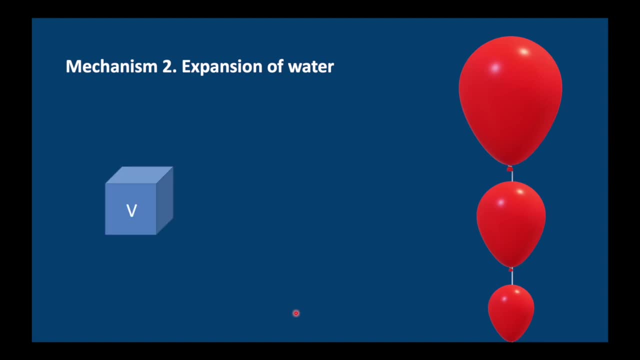 around the outside. Here's a volume of water. We reduce the pressure and it will expand a little bit. Well, not as much as a balloon, of course. In fact, the water compressibility, which is this term called beta, is tiny. It is 10 to the minus 10. 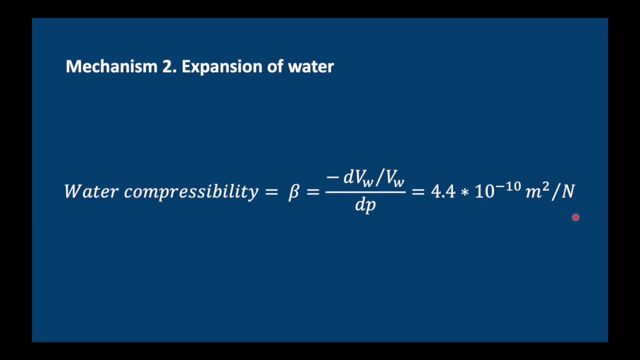 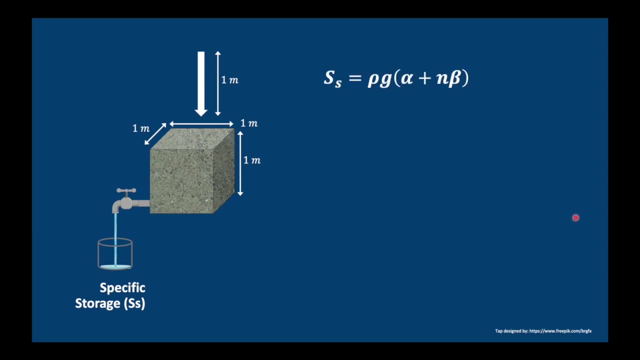 meters squared per Newton, so it's more or less like one of those solid rocks. It does not expand very much. So here's our equation For specific storage, And you'll recognize the alpha term, which is the aqua compressibility, and the beta term, which is the compressibility of water. We 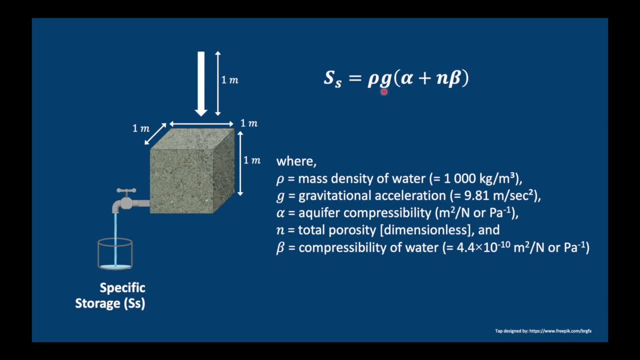 have the density of water, here the gravitational acceleration, and n is the total porosity. This of course depends on your porosity, how much water you have, so these have to be together. Our storativity is the specific storage times by the 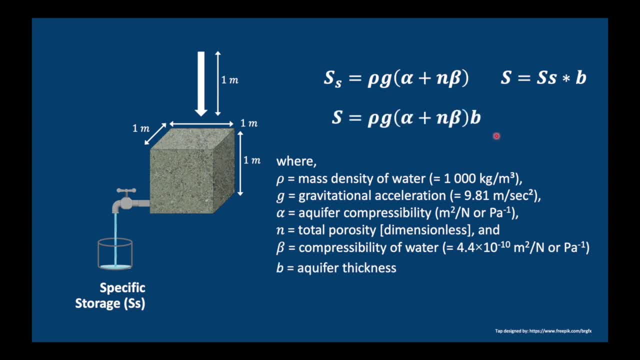 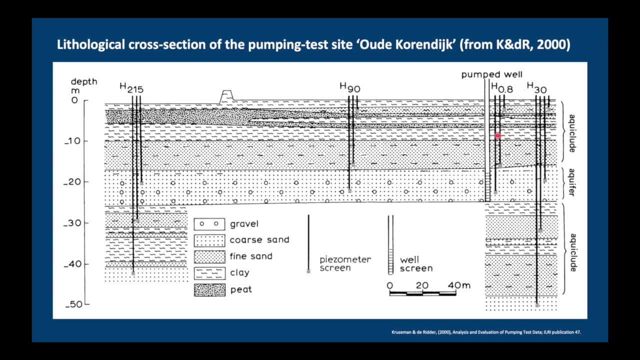 aqua thickness. So here's our total formula. Let's illustrate it with a practical example. This is taken from Krusman and Derrida, the Ode-Kurendijk pumping test, and they have an aquifer thickness of 7 meters. Now this aquifer is made up of coarse. 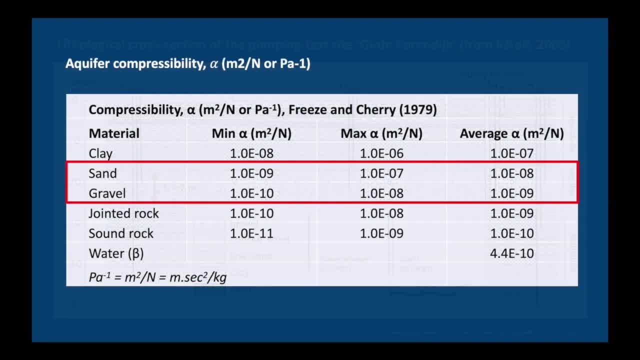 sand with a bit of gravel. If we look at Friesen-Jerry, we can see that the alpha values for sand and gravel is somewhere between 10 to the minus 7 to 10 to the minus 10.. The average temperature is 10 to the minus 8, maybe 10 to the minus 9.. Anyway, we're going to pick one of these. 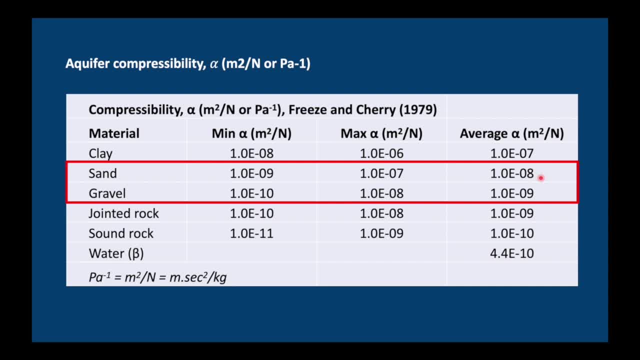 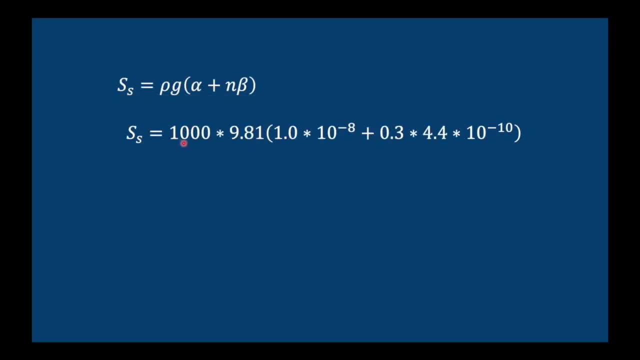 Let's pick 10 to the minus 8, which is kind of the middle range for sand, and we plug it into our equation. This is the weight of water: 1000 kilograms per cubic meter. acceleration due to gravity: alpha 10 to the minus 8.. The porosity we've 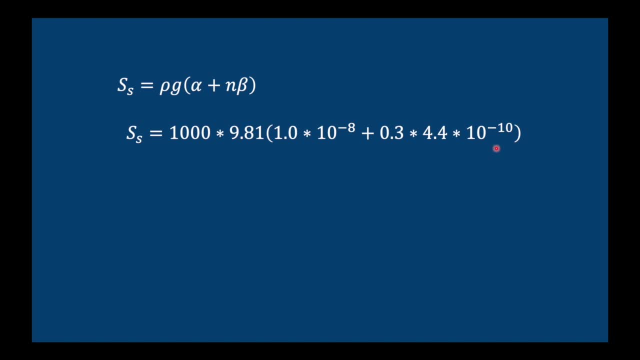 assumed it's 30% or 0.3, and here's our beta term, which is constant. Now this specific storage works out at 9.9 to 10 to the minus 5, and if we times it by the aquifer, 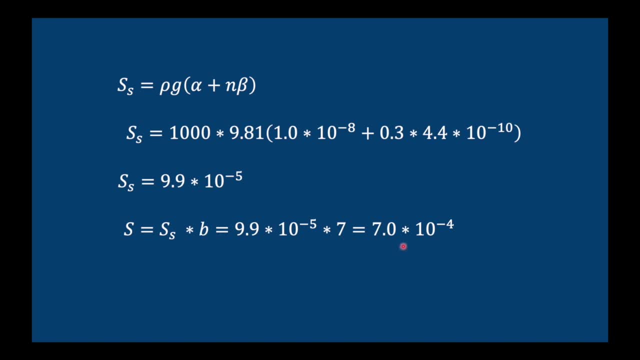 thickness B, which is 7, we end up with 7 to 10 to the minus 4.. Now, when you see 10 to the minus 4, it usually means that we have a confined aquifer and in fact, this is the numbers that we have from the pumping test in. 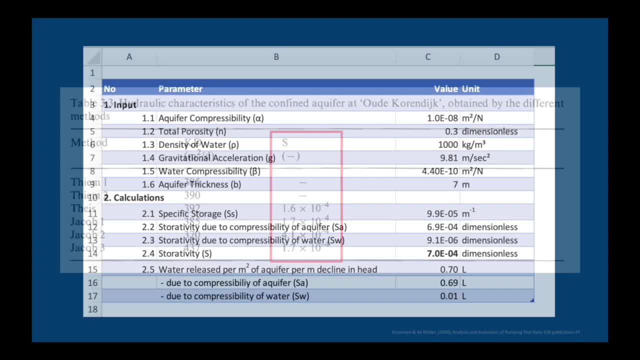 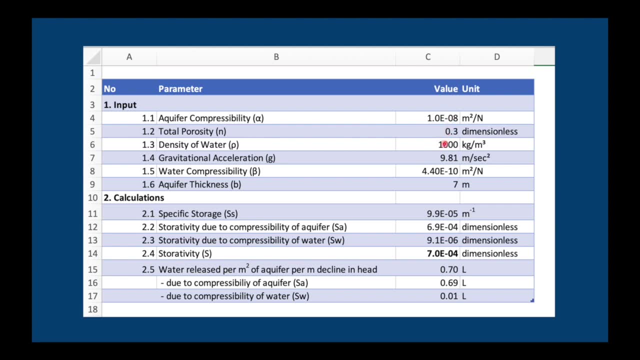 Krusman and Derrida. I've made a spreadsheet where you can do all these calculations automatically. just enter your numbers in here and it will calculate the different specific storage and so on down here. What's quite interesting is, in this example, that per square meter of aquifer 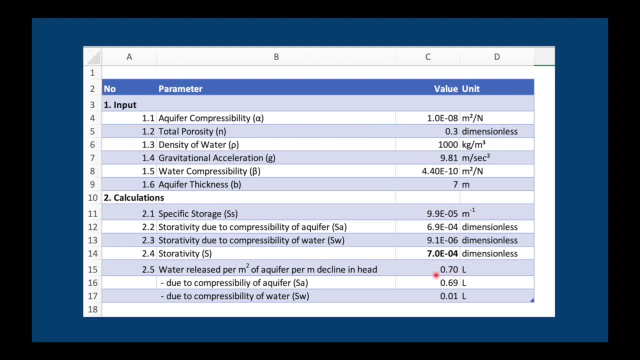 and one meter decline in head. we only get 0.7 liters of water, and most of that water is due to the decompressibility- sorry, due to the compressibility of the aquifer rather than the compressibility of water. 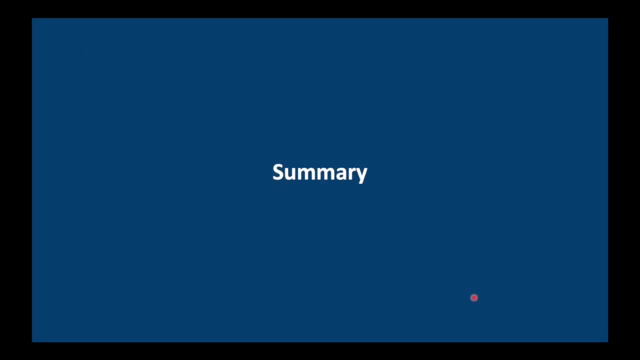 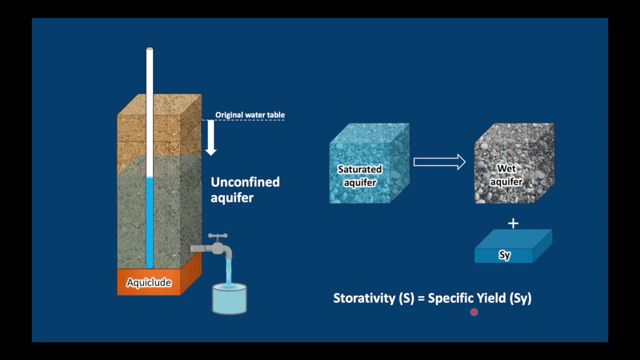 Ok, in summary, in our unconfined aquifer, our storativity is the same as our specific yield, which means it is the amount of water that can drain under gravity from the saturated aquifer. In confined aquifers we have to consider.